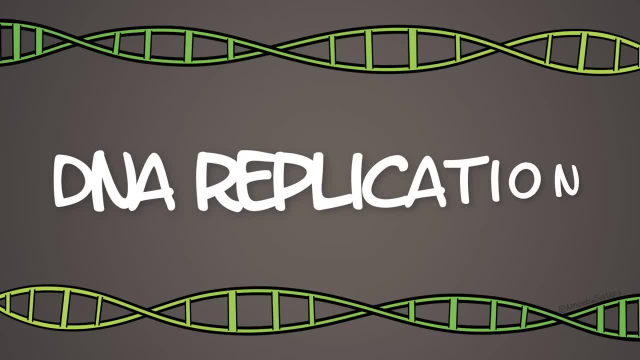 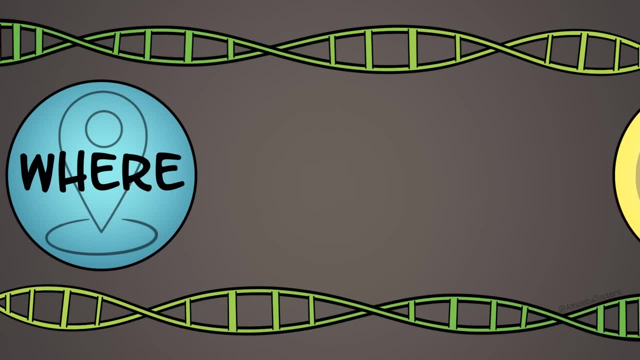 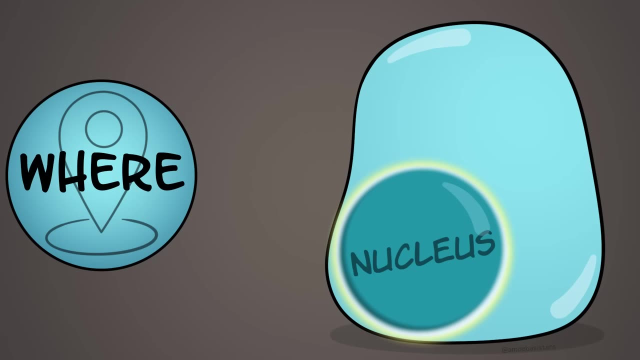 new daughter cell. And that introduces our topic of DNA replication, which means making more DNA. First let's talk about where and when. First, where? Well, if it's in a eukaryotic cell, it occurs in the nucleus. However, remember, not all cells have a nucleus. 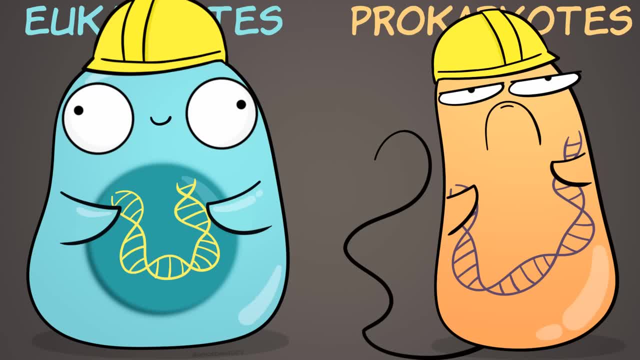 Such as prokaryotic cells. They don't have a nucleus. Still, both prokaryotic and eukaryotic cells do DNA replication, but there's some differences between the two that this clip doesn't go into. Next, when, When does this happen? Well, a cell is going to need to do. 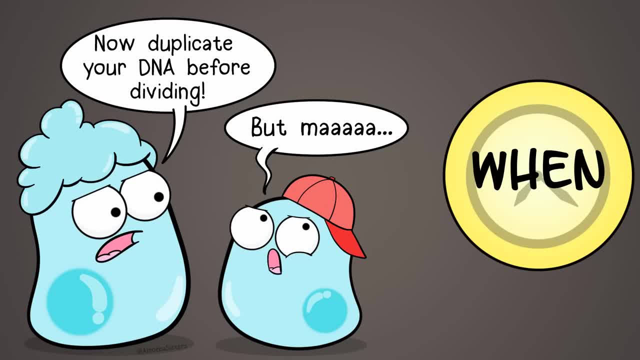 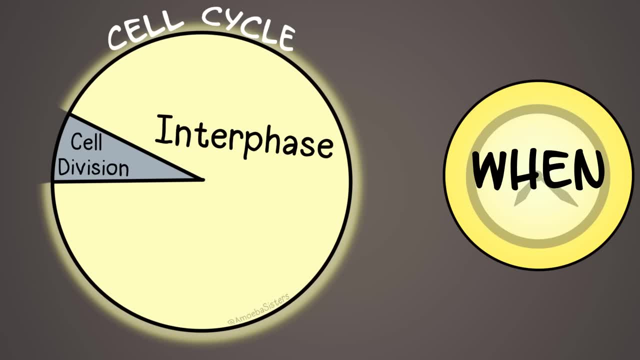 this before it divides, so that the new daughter cell can also get a copy of DNA. To get specific, in a eukaryotic cell that's going to be before mitosis or meiosis, in a time known as interphase, I think DNA replication would. 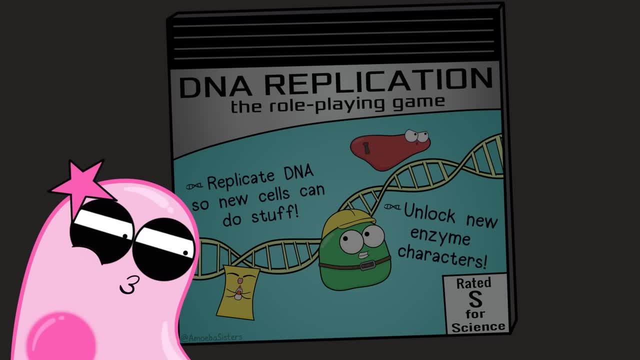 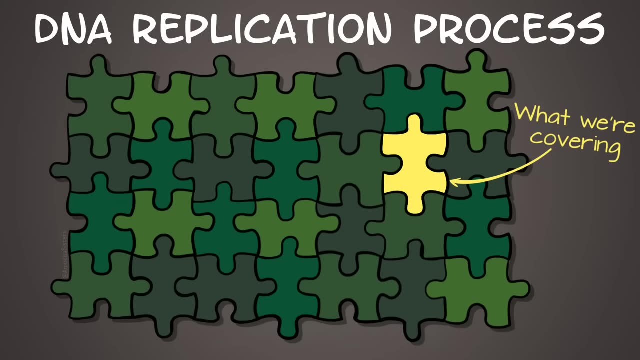 actually make a great video game. Still waiting for that to be invented, I'm going to introduce the key players in DNA replication so that you can get some background information Now. remember, these are just some major key players. There's a lot to this process. 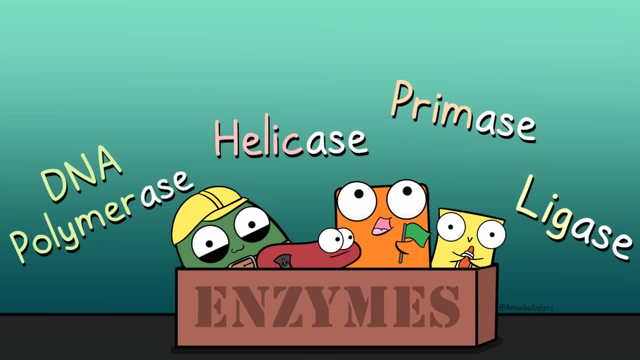 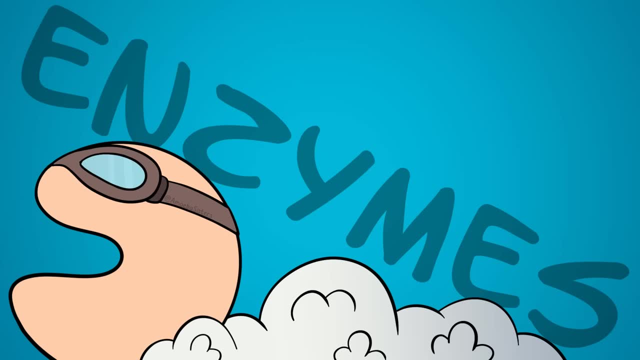 Many of the key players are enzymes In biology. when you see something end in A-S-E, you might want to check, as it's very possible that it's an enzyme. Enzymes have the ability to speed up reactions and build up or break down the 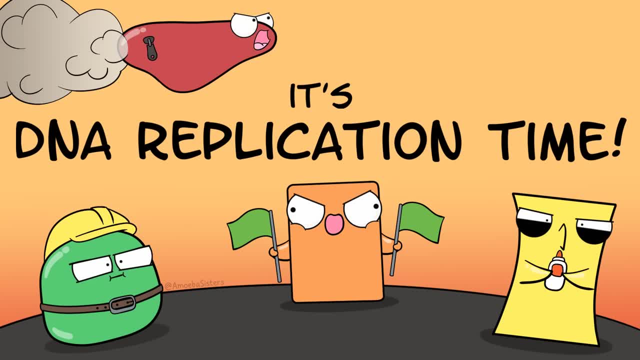 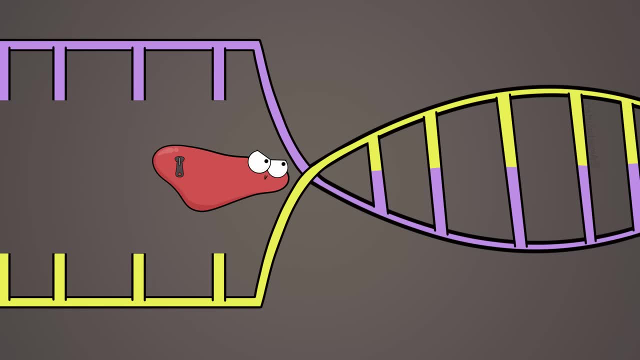 items that they act upon. So here we go with the key players: Helicase, the unzipping enzyme. If you recall that DNA has two strands, you can think of helicase unzipping the two strands of DNA. Helicase doesn't have a hard time doing that When unzipping it breaks through. 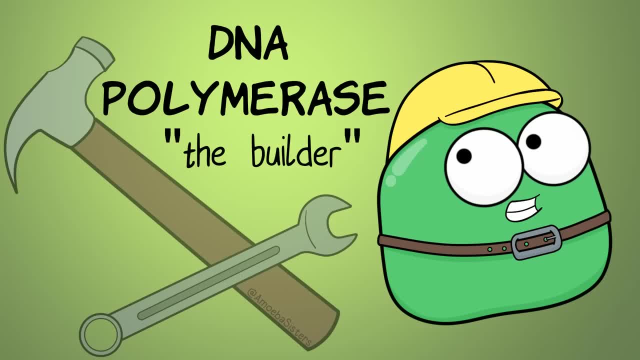 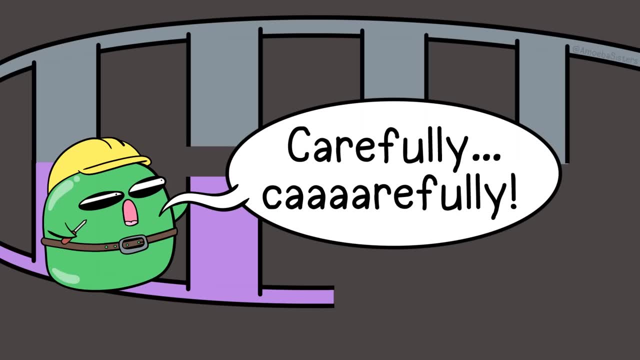 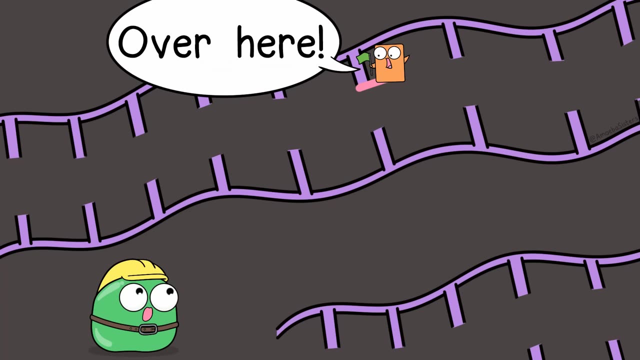 the hydrogen bonds that hold the DNA bases together. DNA polymerase, the builder: This enzyme replicates DNA molecules to actually build a new strand of DNA Primase, the initializer. With as great as DNA polymerase is, DNA polymerase can't figure out where to get started without something. 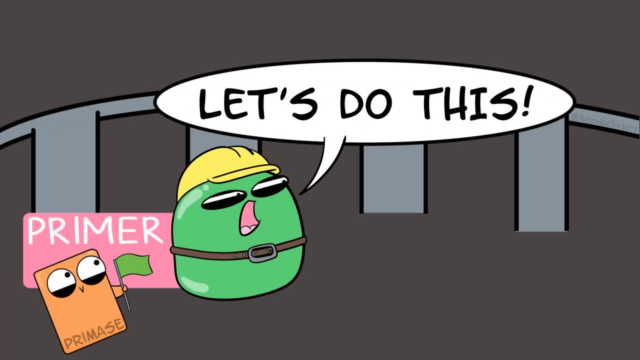 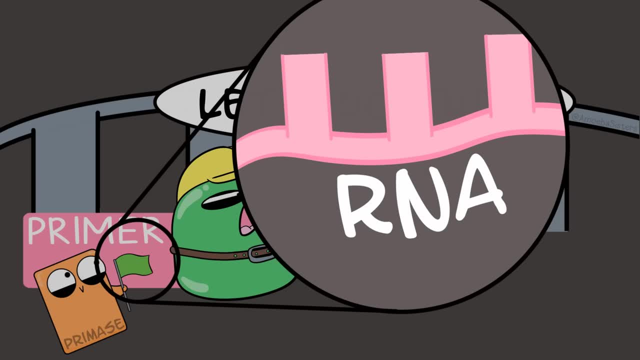 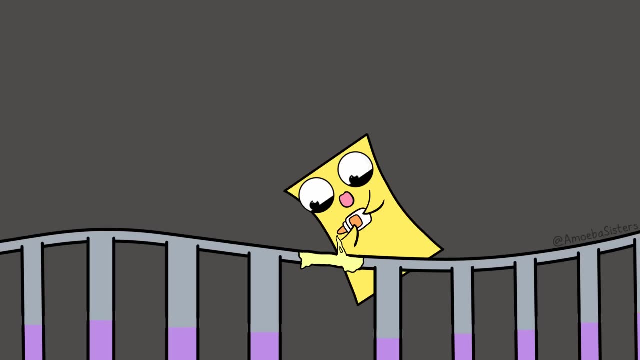 called a primer. Primase makes the primer so that DNA polymerase can figure out where to go to start to work. You know what's kind of interesting about the primer it makes? The primer is actually made of RNA Ligase, the gluer. It helps glue DNA fragments together. More about why you would need that. 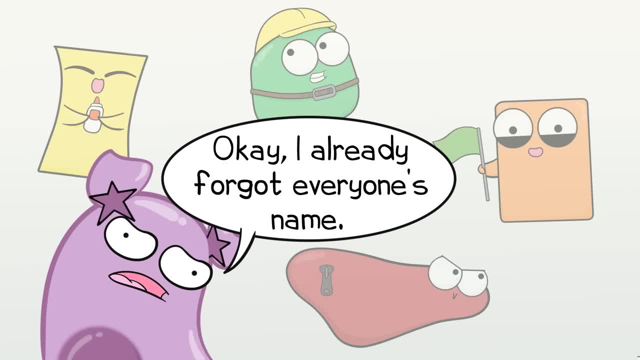 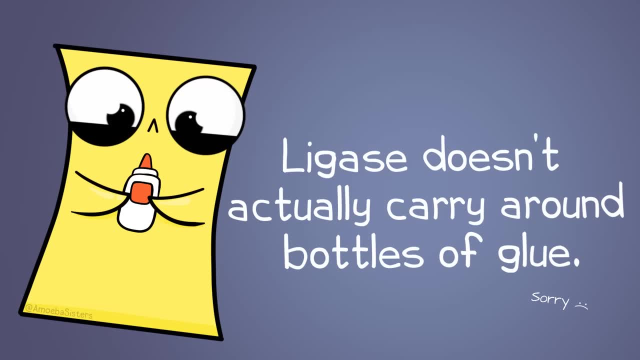 later on. Now don't feel overwhelmed. We'll go through the basics of this sequence in order, But remember, like all of our videos, we tend to give the big picture. There are always more details and exceptions to every biological process that we can't include in such a 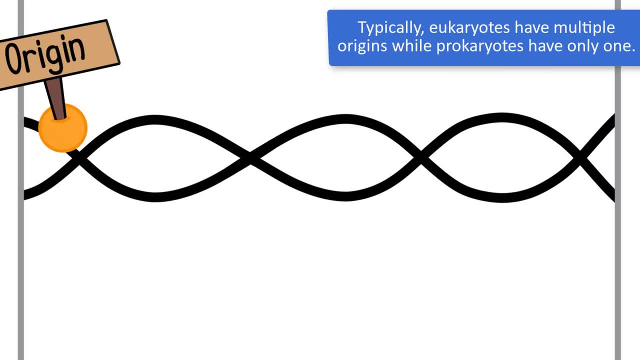 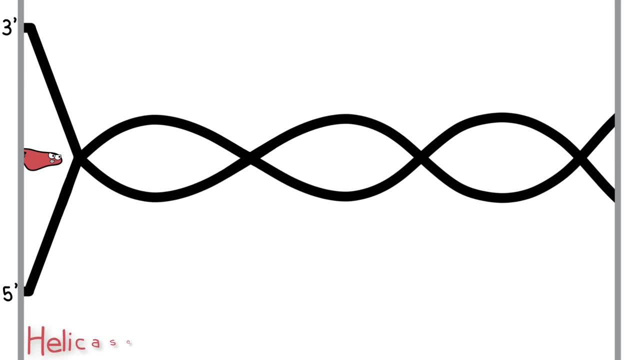 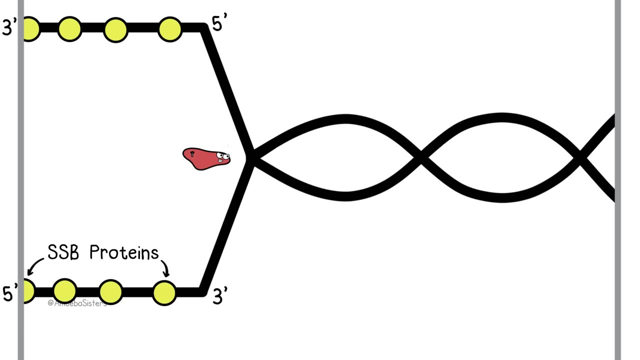 short video. DNA replication starts at a certain part called the origin. Usually, this part is identified as the origin. At the origin helicase, the unzipping enzyme comes in and unwinds the DNA. Here's the thing, though. you don't want these strands to come back together. 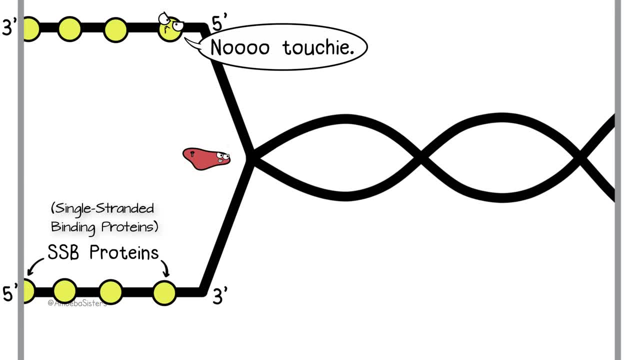 So SSB proteins, which stands for single-stranded binding proteins, bind to the DNA strands to keep them separated- And topoisomerase. I always have to slow down when I say that enzyme's name keeps the DNA from supercoiling. Supercoiling might sound super and it can be when you're. 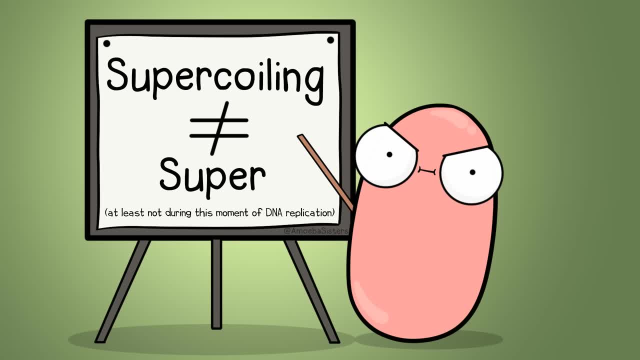 trying to compact the DNA, but it's something that needs to be controlled during the process. So what is supercoiling? Well, it's something that keeps the DNA from supercoiling. Supercoiling can be controlled during DNA replication. Supercoiling can involve an overwinding of 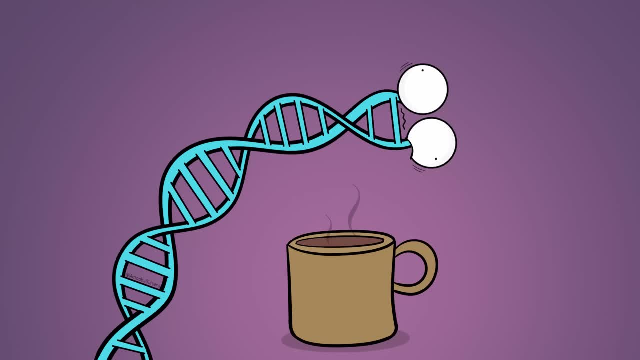 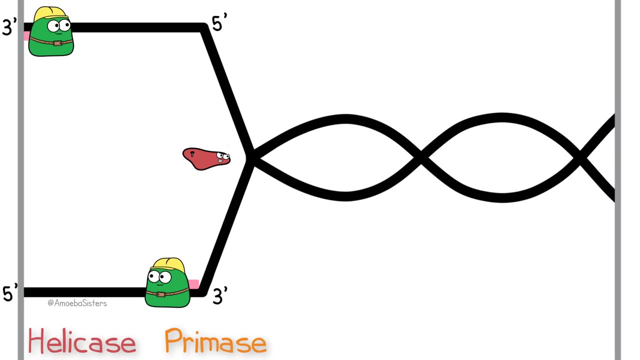 the DNA and you need the DNA strands to be separated for the next steps. Primase comes in and makes RNA primers on both strands. This is really important because otherwise DNA polymerase won't know where to start. In comes DNA polymerase. 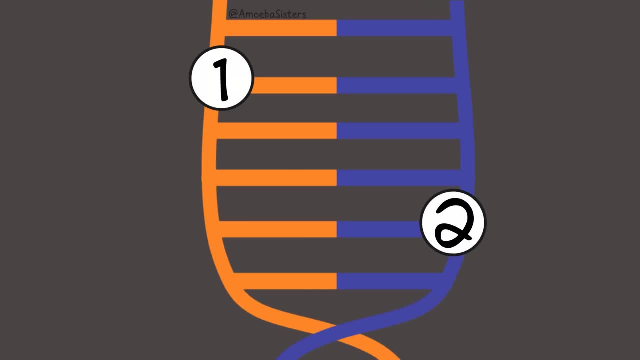 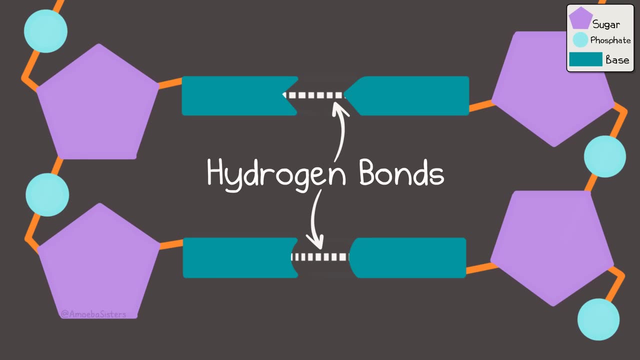 Ok, before we go on, remember how we said: DNA has two strands. They're not identical, they complement each other. In our video that covers DNA structure, we talk about how the bases pair together with hydrogen bonds. The base adenine goes with the base thymine. 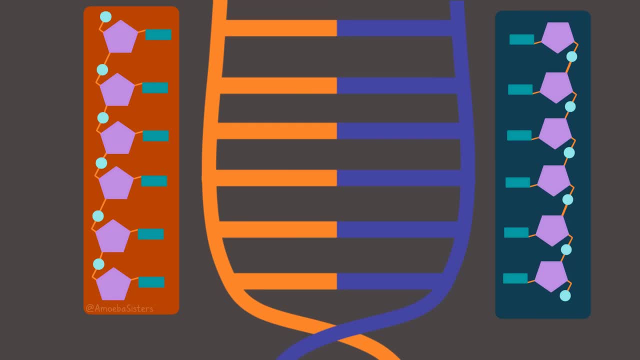 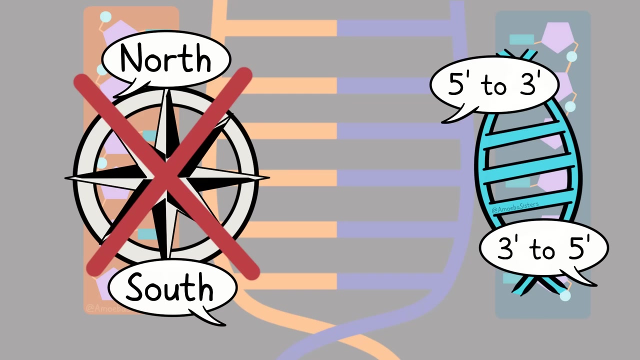 and the base guanine goes with the base cytosine. These strands are also anti-parallel, so they don't go in the same direction. What do we mean by direction? Well, with DNA we don't say north or south, We say DNA either goes 5' to 3' or 3' to 5'. What in the world? 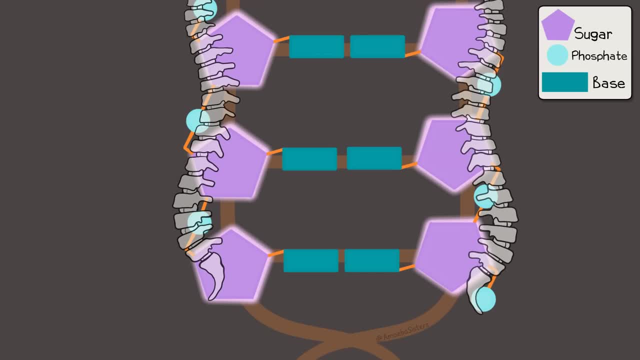 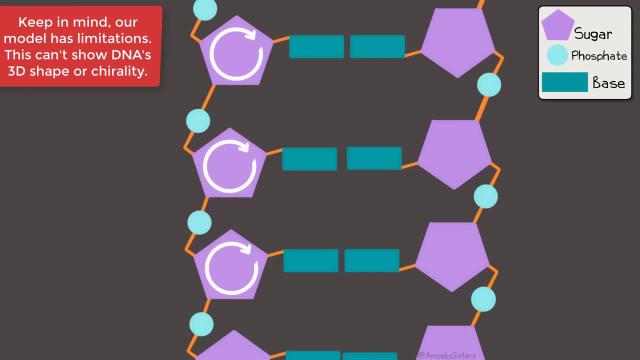 does that mean The sugar of DNA is part of the backbone of DNA? It has carbons. The carbons on the sugar are numbered right after the oxygen in a clockwise direction: 1', 2', 3' 4' and. 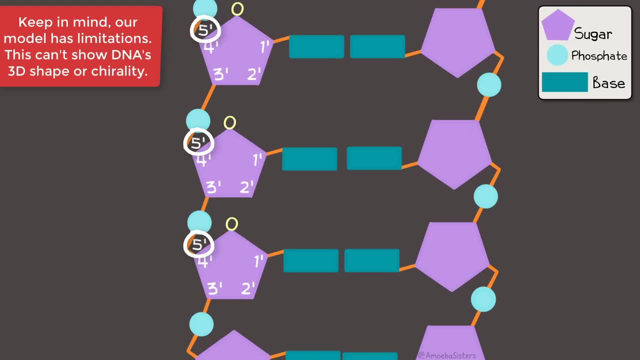 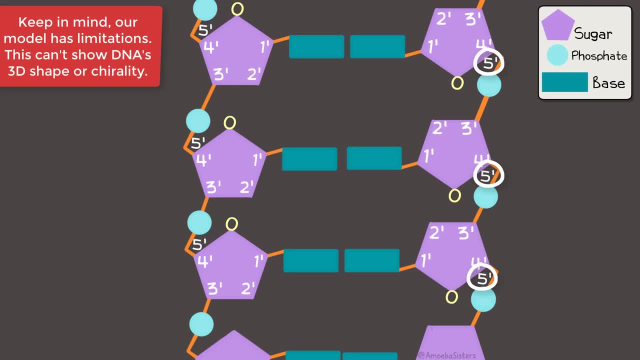 4', 3' 4', 3', 4', 3', 3', 4', 3', 4�. This strand on the right runs 5' to 3', and the strand on the left here runs 3' to. 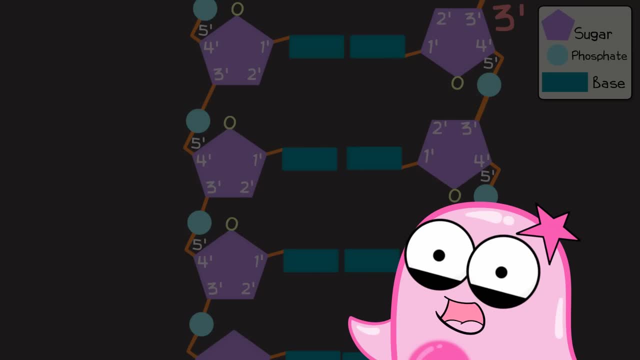 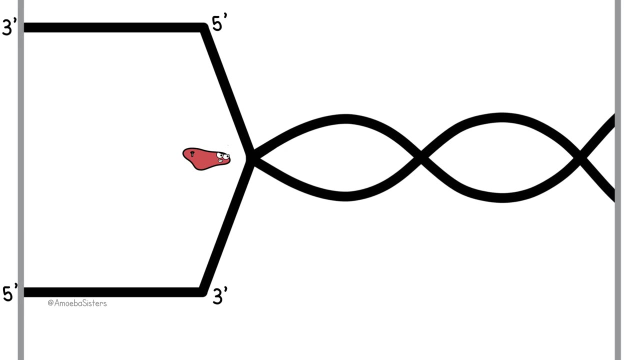 5'. We'll explain why all of that matters in a moment. So let's take that knowledge there and look at DNA replication here. In this image I labeled the top original strand 3' to 5'. I labeled this bottom original. 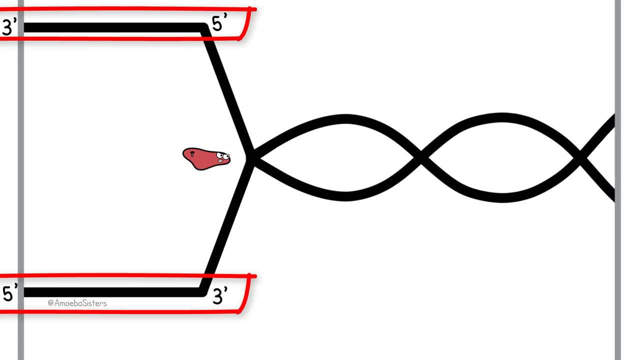 strand 5' to 3'. That's the original DNA that is not aligned on the right side. What's going on here is the original simple DNA has two parts. calling going to be replicated. DNA is unwinding here thanks to helicase. 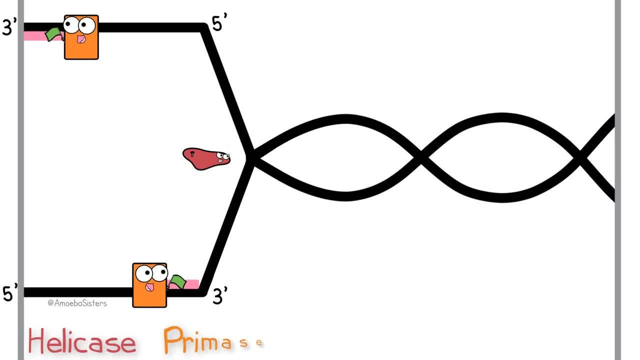 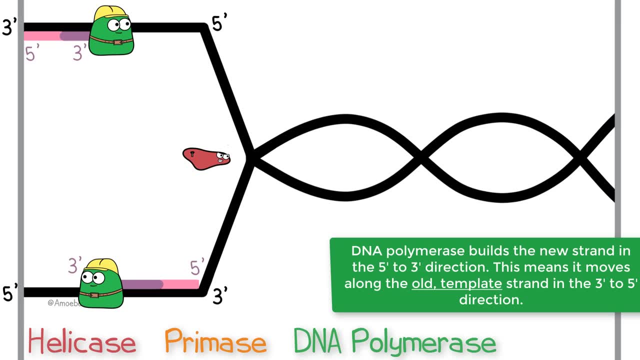 In this example, it will keep unwinding in this direction. Primase places primers. DNA polymerase is building the new strands. Now the thing about DNA polymerase is, when it's building a new strand, it can only build the new strand in the 5' to 3' direction, meaning it adds new bases to the 3' end. 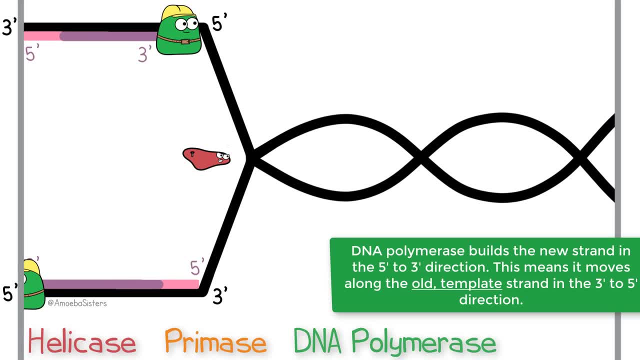 on the new strand. See how it's being built in the 5' to 3' direction. This one is called the leading strand, But take a look down here. So DNA polymerase, once again, is building a new strand in the 5' to 3' direction. 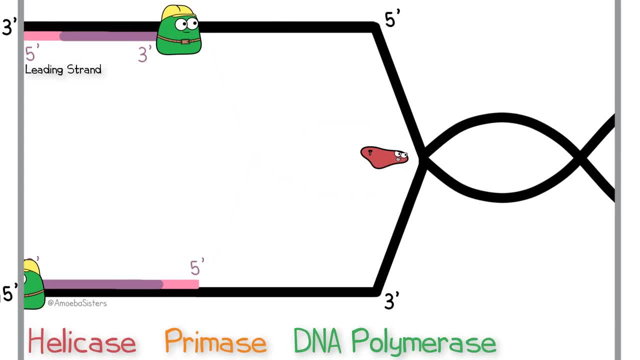 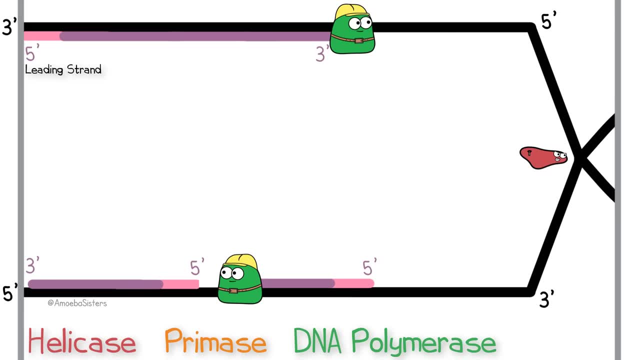 But there is a bit of a problem here. See as DNA unwinds, because DNA polymerase can only build the new strand in the 5' to 3' direction. it has to keep racing up here, next to where this unwinding is happening. 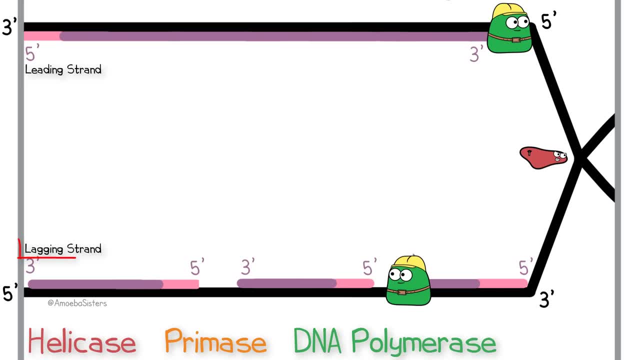 You can see why, then, this new strand is new. In order to build the new strand, the primary elements are called the lagging strand. On this lagging strand, primers have to keep being placed in order for DNA polymerase to build.